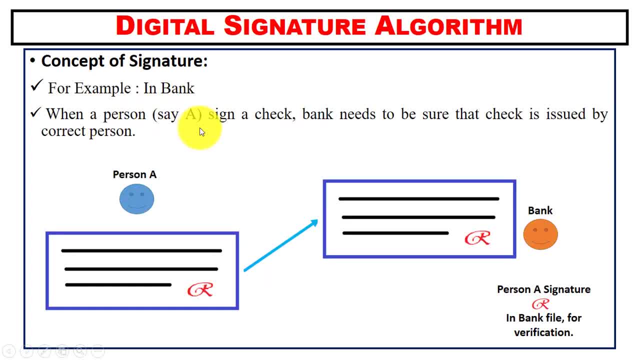 For example in bank, when a person, suppose A this person- signs a check, now bank needs to be sure that the check is issued by the correct person. So in this case this person's signature verification is done by the bank. Signature matched check is accepted, else rejected. 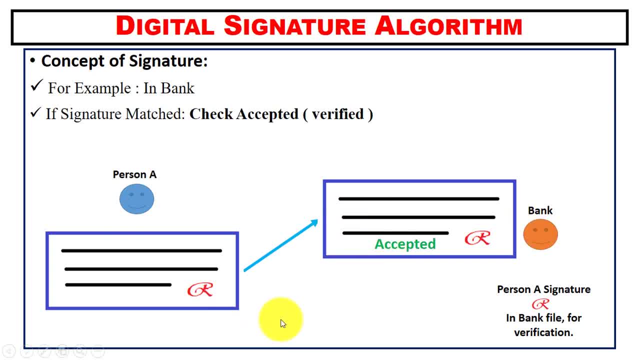 So in this case you can see on the check the signature. On the check we have a signature and you can see in the record we have another signature of this person. So when the person's signature is matched then check is accepted. It means signature verified. 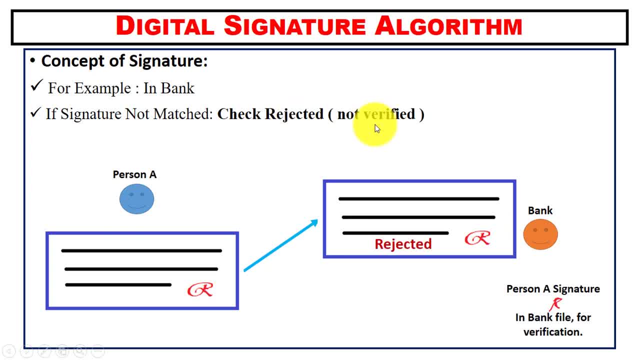 If this signature is not matched, it means signature is not verified, So check is rejected. Suppose in this case we have a signature on the check you can see here and in the record we have another signature. So in this case signature is not matched, So check is rejected. 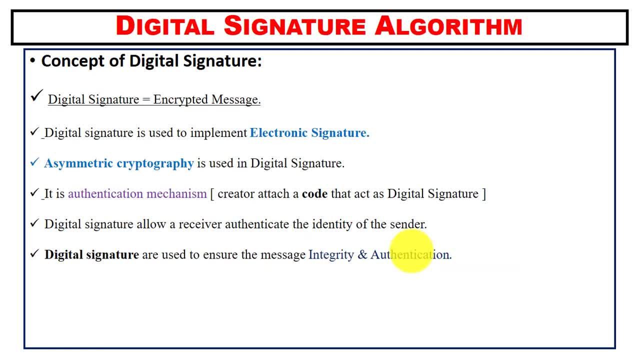 Same concept we are using here in digital signature, but in this case there is a little bit difference, As in case of digital signature, we are using here electronic signature instead of this. So now we have electronic signature. That is nothing, Just the code that is attached by the creator that act as a digital signature. 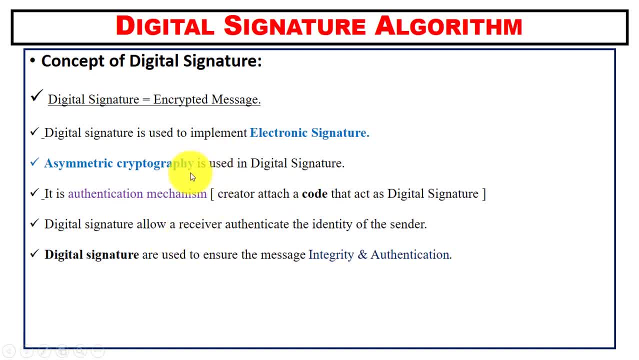 So here digital signature is the encrypted message and we are using here for the authentication mechanism. using digital signature, Receiver can authenticate the identity of the sender and the integrity of the message. here We are using asymmetric cryptography in the digital signature. It means we are using asymmetric key. 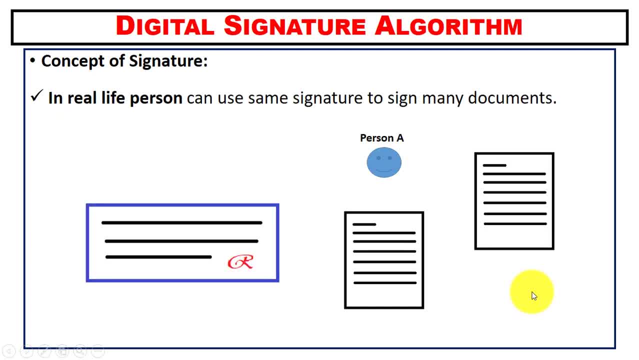 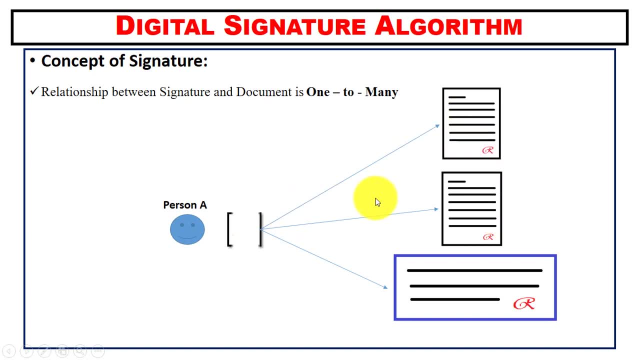 That is the public key, The public and the private keys for the encryption and the decryption. in real life person can use same signature to sign many documents. As you can see, we have a person, a, and you can see this person can use same signature on many documents. 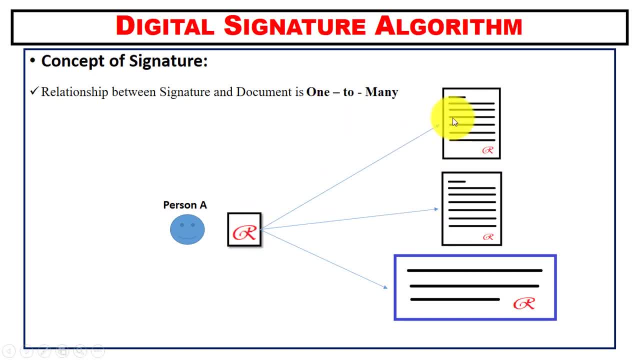 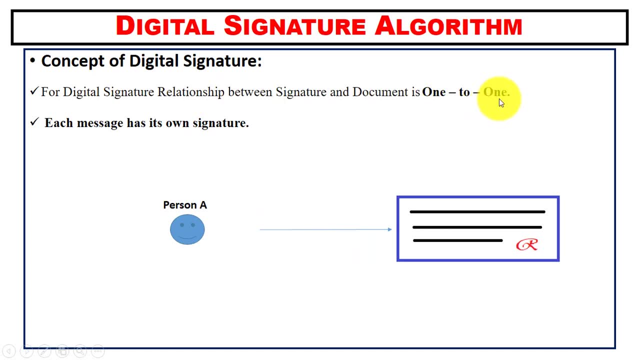 That is the relationship between the signature and document- is one too many. That is, one signature can be used to sign Many documents in real life, but in case of digital signature, you cannot use same signature to sign many documents. so you cannot use the same signature to more than one document. 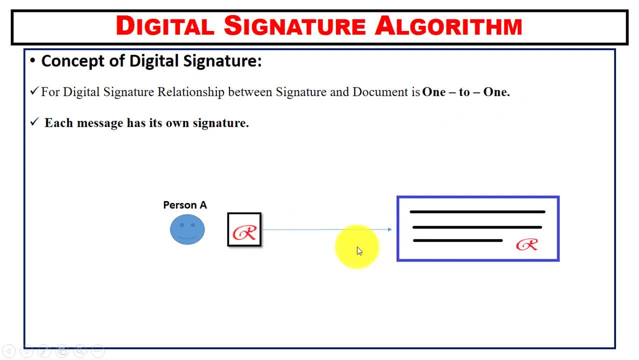 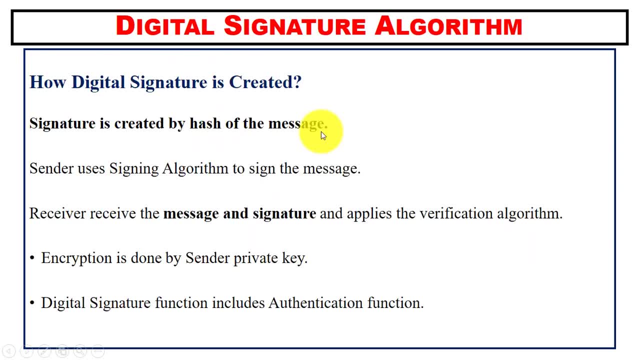 So in this case, the relationship between the signature and the document is one to one. Each message has its own signature. done So, how digital signature is created? This is created by the hash of the message, And here sender uses signing algorithm to sign the message and when the receiver will receive the message and the signature verification algorithm is applied in order to check the authentication. 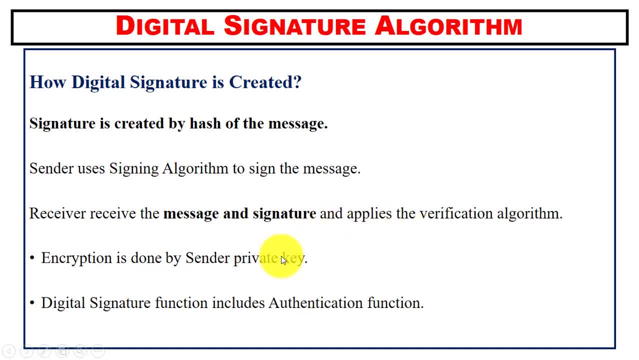 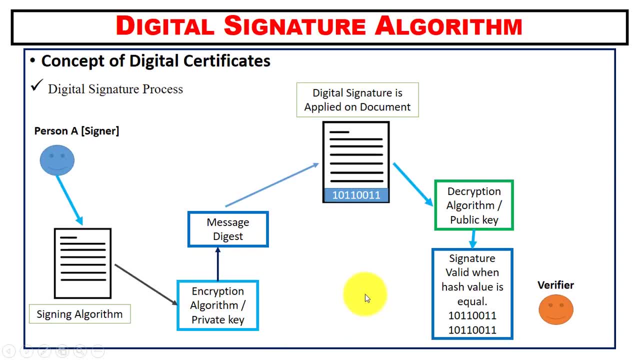 After that you can see encryption is done by the sender private key. So this is the process, how digital signature is working. So suppose we have sender A, That is the Signer, and we will use here signing algorithm to sign the document. 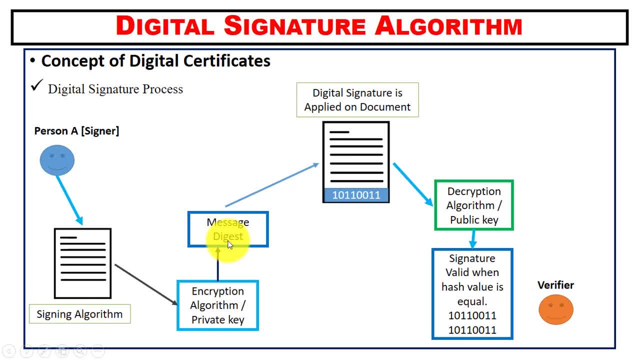 After that, encryption is applied and message digest is generated And you can see: this is the digitally signed document. or you can say: digital signature is applied on this document. Now you can see here, the code is attached here. After that, We will apply the verification algorithm for the verification purpose. 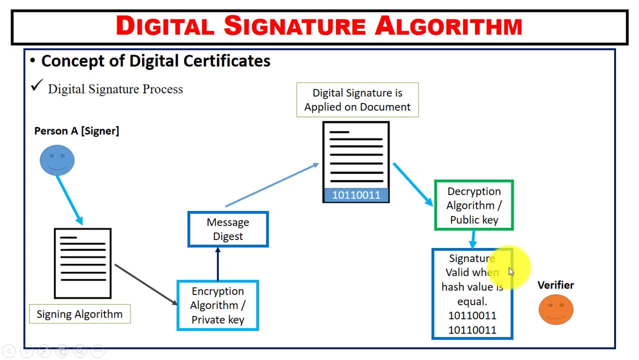 First we will decrypt the message. So decryption algorithm is applied here. We will check the hash code that is generated here. If the hash value is equal, then signature is valid, else not. So in this case, verifier will check the hash value that is generated. 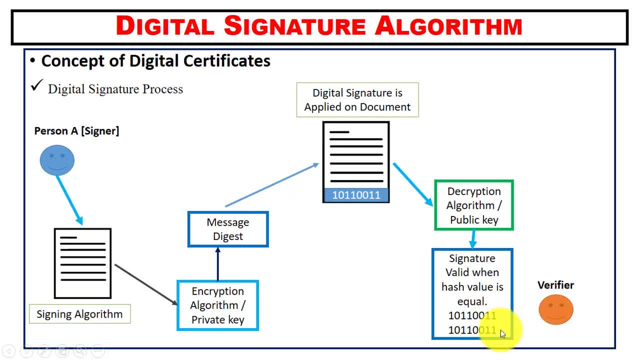 If the value is matched, it means signature is verified, It comes from the authenticated entity. So in this case, you can see, we can use this algorithm to verify when the message comes from the verified entity or not. So this is the simple algorithm we are using here.